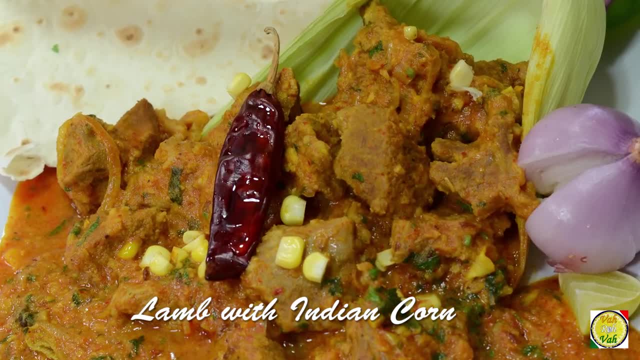 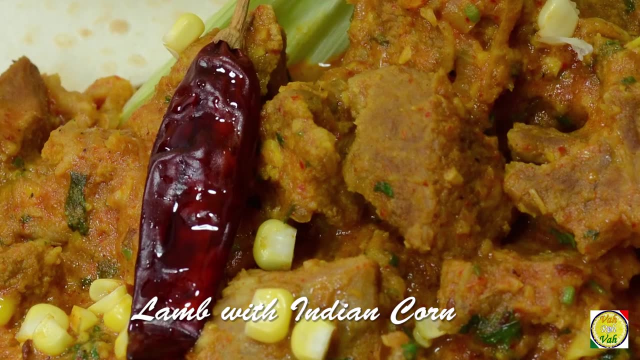 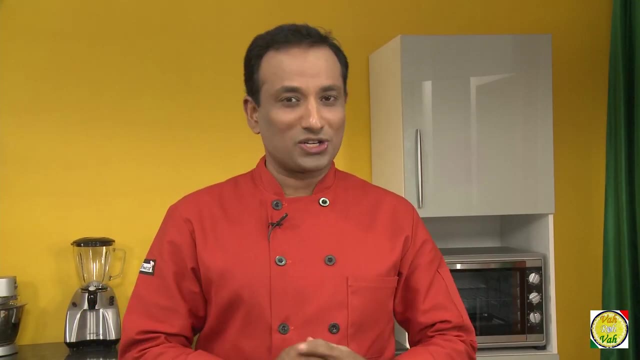 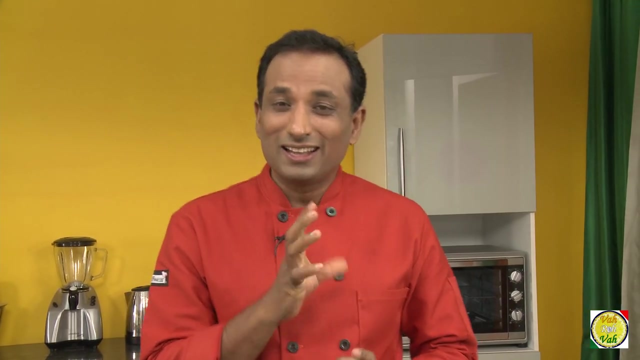 hello namaste salaamwalekum satsriyakaal, welcome back to another session with your VahChef at Vahrehvahcom. Today I'm going to copy a recipe and make it my own. this is a kind of a Rajasthani preparation, where they use makai and 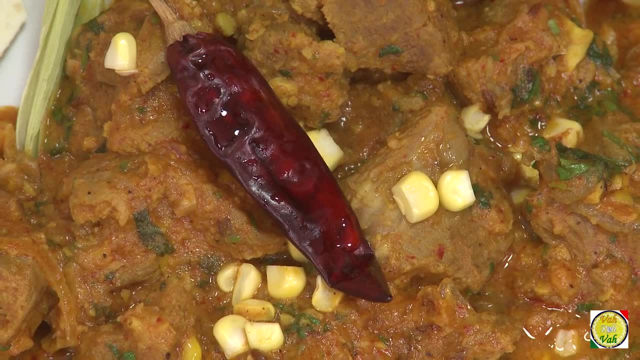 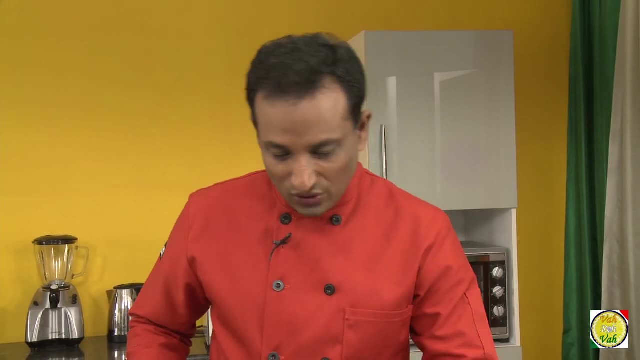 cook lamb with it. it's usually, I think, the name is called makai ka soya ta, but today I'm going to make small subtle changes and make this dish. so first for this dish, add ghee in a pan. in this, add whole garam masala, add jeera. 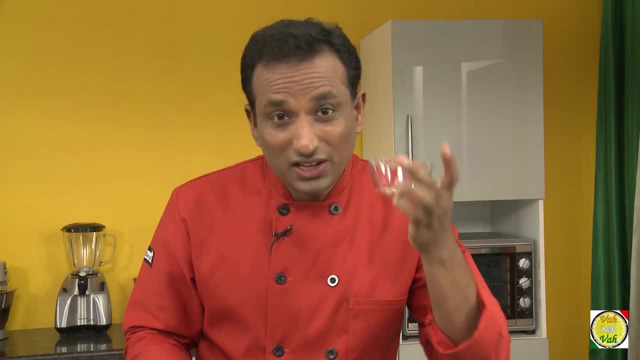 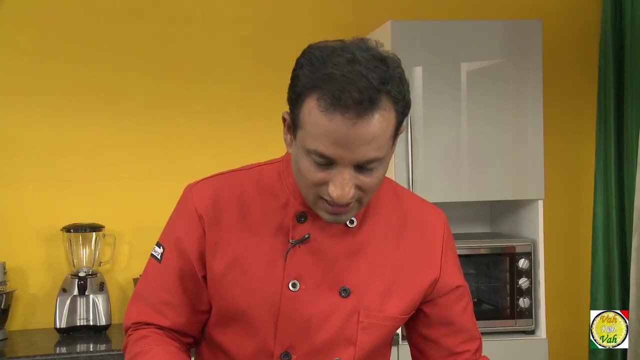 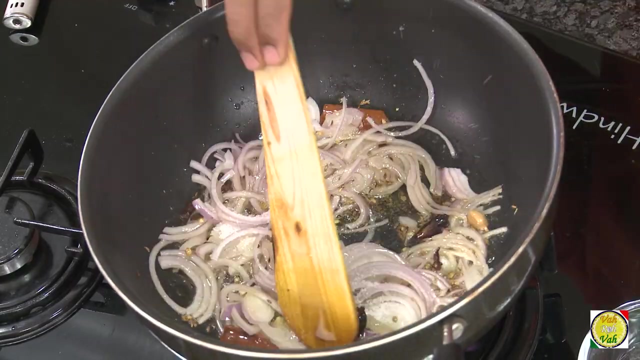 chai jeera. we're going to add crushed dhaniya. as soon as you add dhaniya, you're going to add slice of onions. here is a crushed dhaniya and this add slices of onions, add salt and we're going to cook this till these onions are slightly golden in. 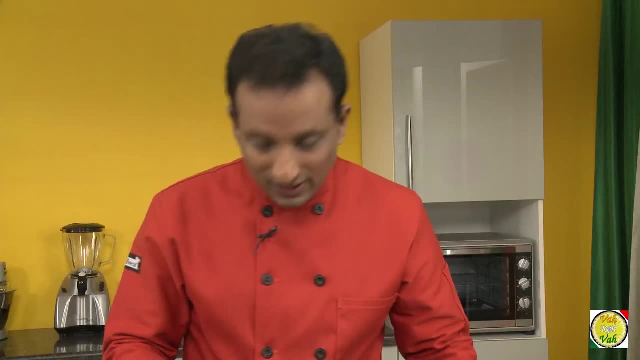 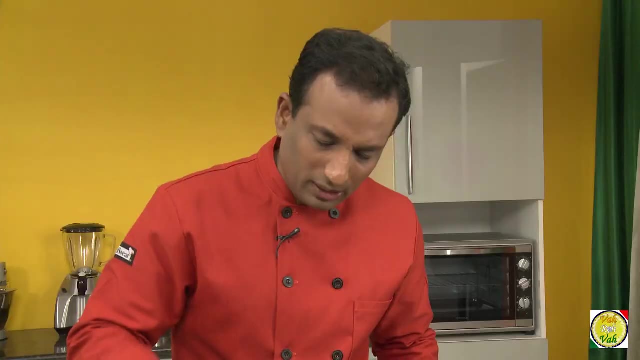 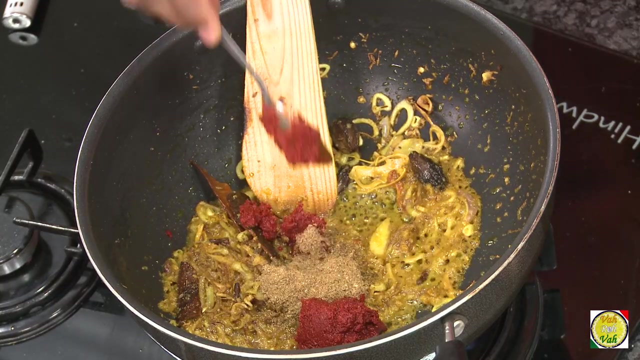 color. now add mace, that is javitri. add turmeric ginger garlic paste. you know, just cook this ginger garlic paste little bit, not too much. add coriander powder, red chili powder- or I have lot of red chili paste. this is going to give. 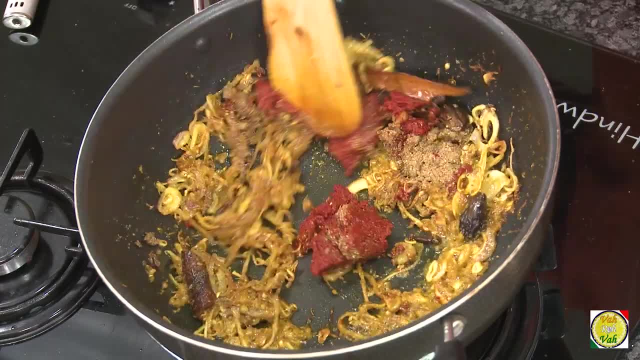 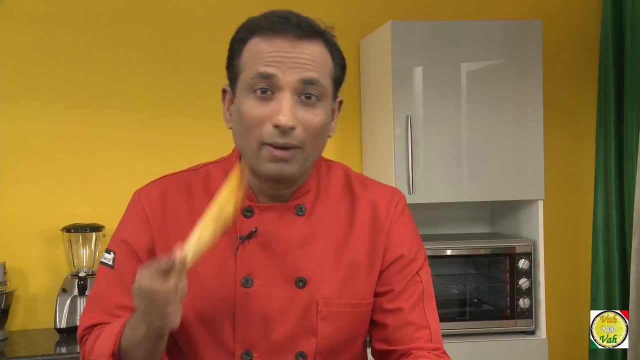 lot of nice color, so I'm going to add some red chili paste and switch off the flame. I forgot to add bay leaf, so I'm going to add bay leaf. now. add mutton, mind you, I switched off the flame. ok, then add mutton and little bit of garam. 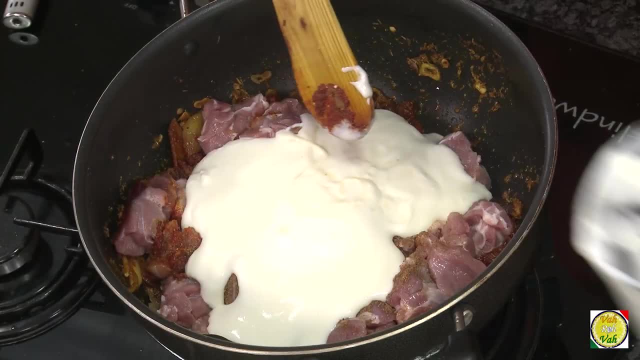 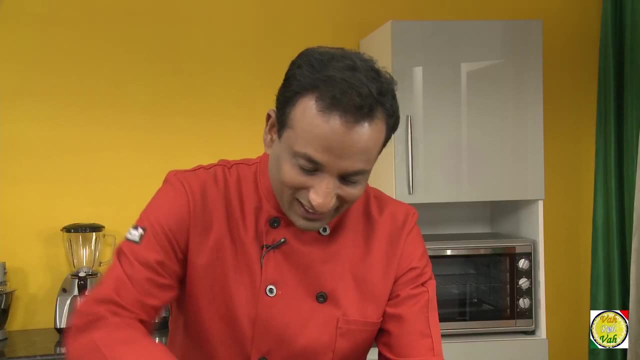 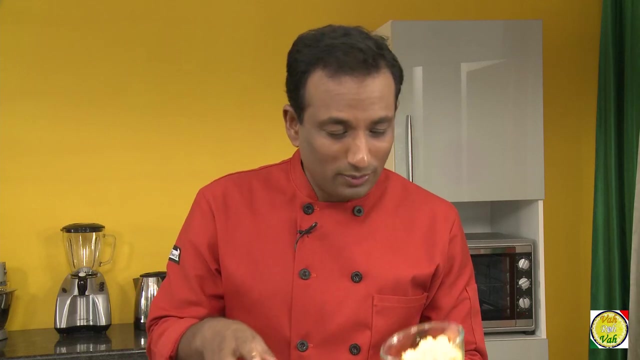 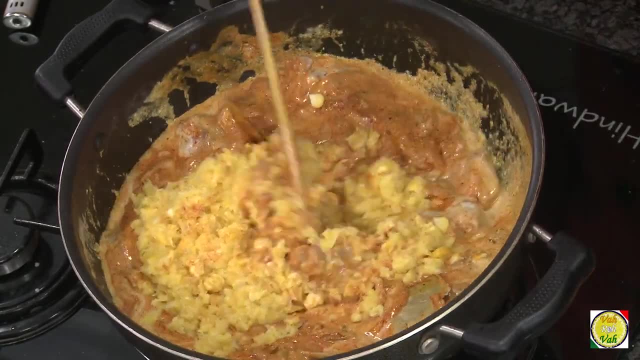 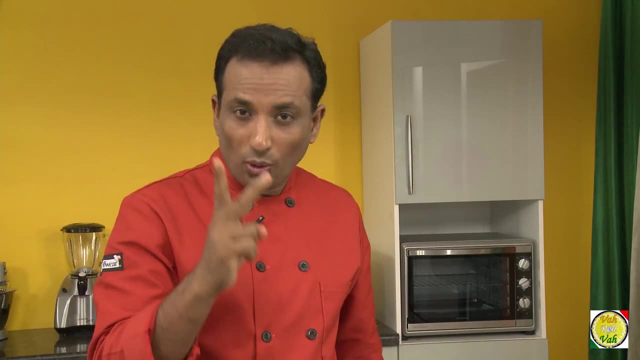 this is the corn from India, what we call butta. so I just, you know, put it in a blender, crushed it and added to this. now we're going to rest this meat for two hours. ok, just put the lid. you remember I switched off the flame even before I. 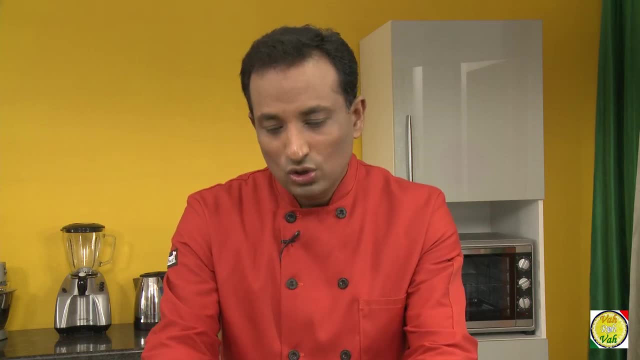 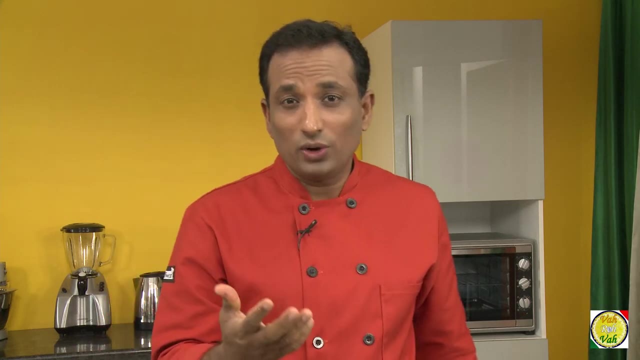 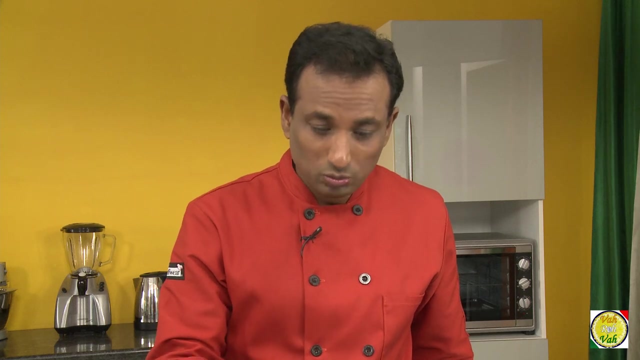 put the mutton. so this is not hot at all. so we're going to let this marinate for two hours and later put it on the stove and cook it. if you want to do it overnight now, you can put this in the refrigerator and cook it the next day morning, but I'm just going to leave it aside for two. 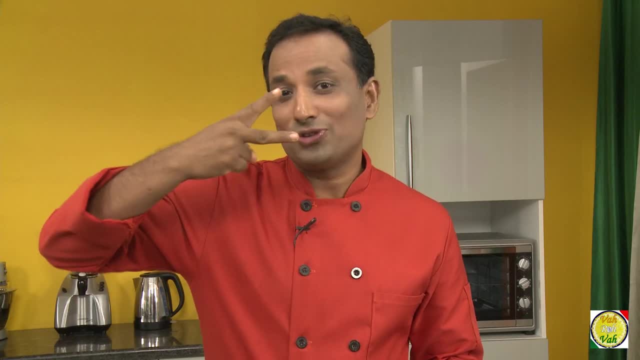 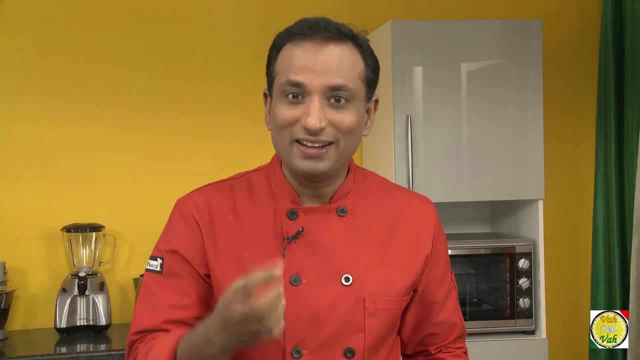 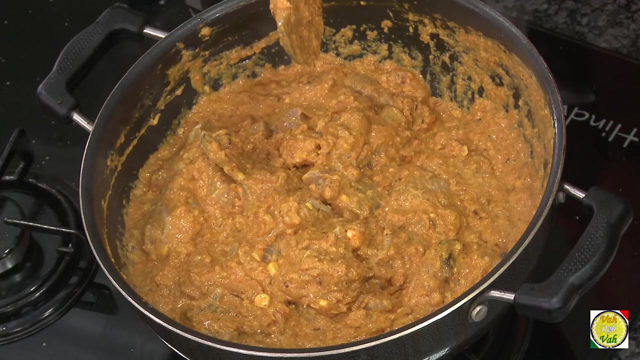 hours, then I'm going to start the cooking process now. after two hours, I'm going to light this stove and I'm going to cook this till the meat is nice and tender. you know, while cooking till this comes to a boil, keep mixing, otherwise it will burn at the bottom. 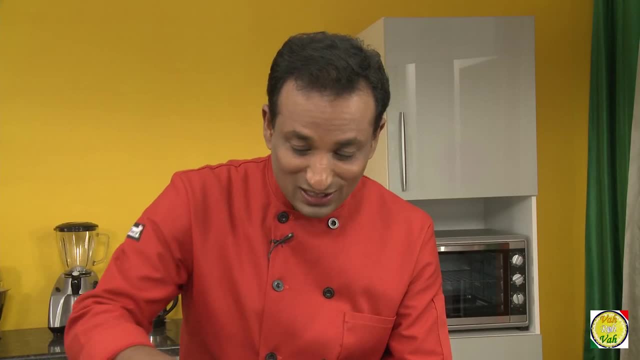 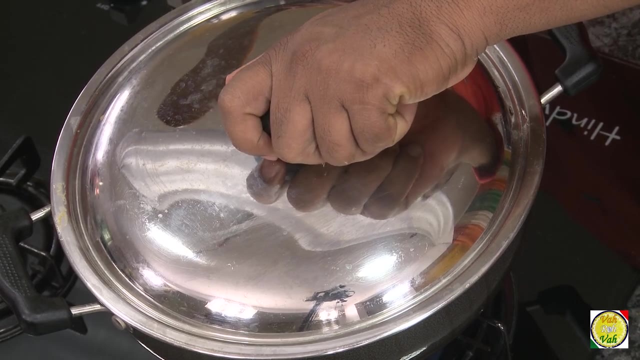 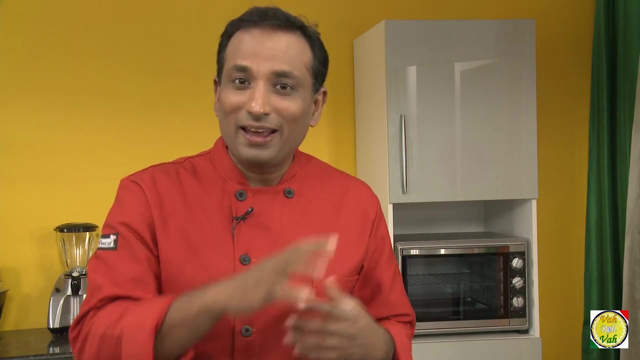 so be very careful. slowly the mutton will lose out water and this will become a very nice gravy, wow. so keep cooking till the meat is nice and tender. this recipe is like one Hyderabadi trespassing Rajasthan. see, in Rajasthan, when they marinate meat, they just marinate with yogurt and other spices. 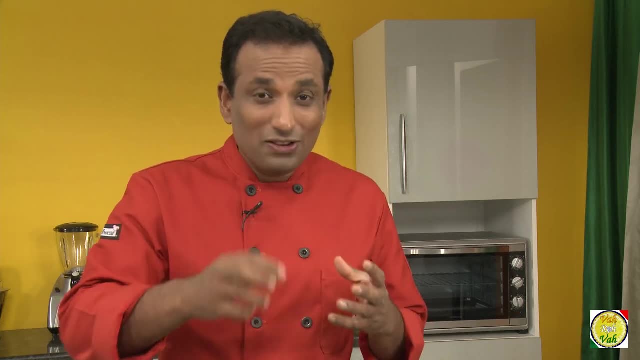 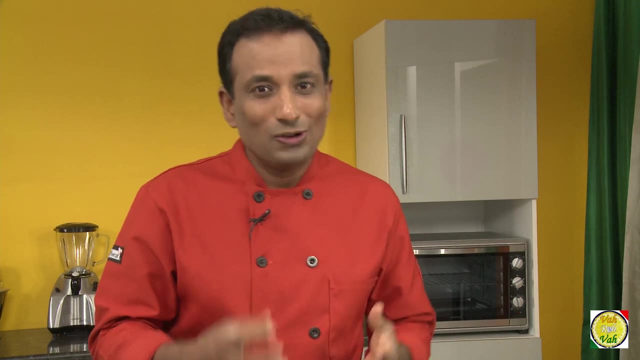 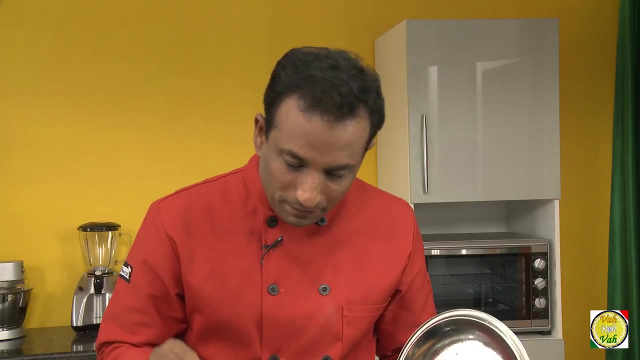 but we in Moghalai cooking, what we do is we fry onions, we fry masalas and then marinate it so that way to extract more flavor from it. so, whatever it is, the end result is going to be awesome. look at this. you know it is a slowly reducing. you can add water if this is. 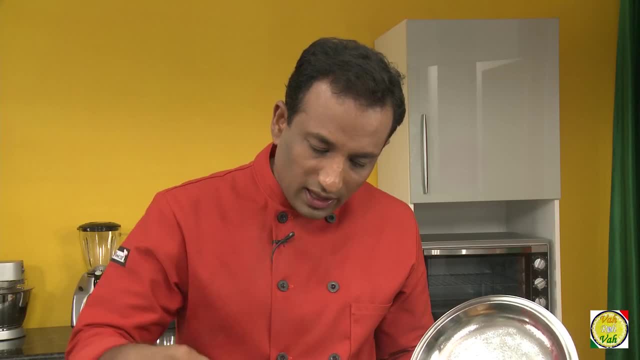 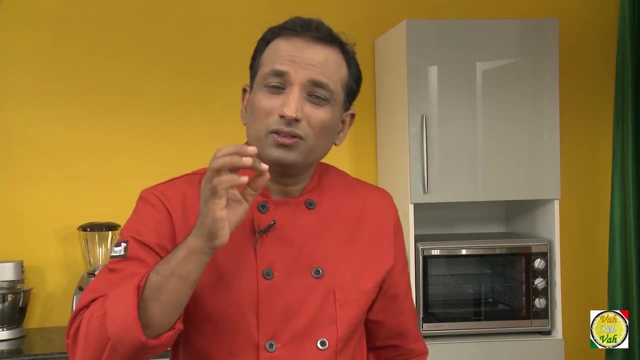 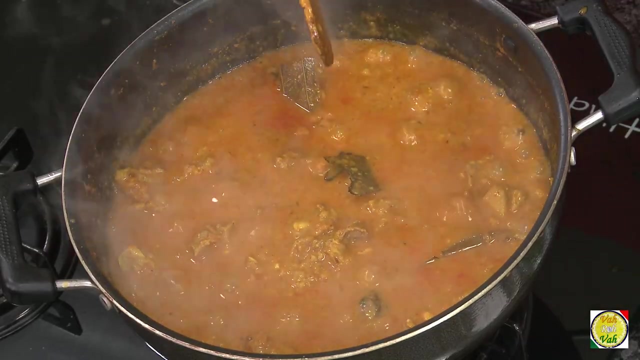 getting thicker. so I added a little bit of water and keep cooking till the meat is nice and tender and put the lid on and slowly cook for another 15 minutes. so far I have cooked for almost 20 minutes. another 15 minutes should be good. Now you know. look at this consistency of the sauce, this corn, not 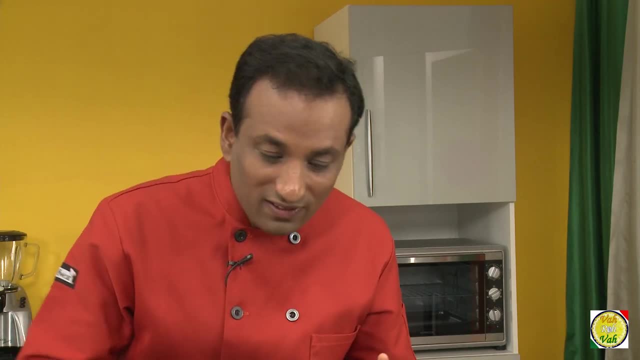 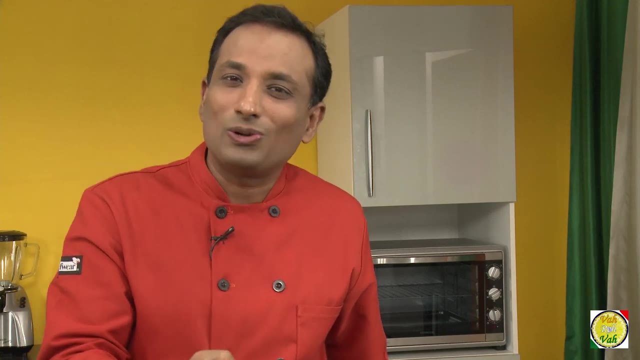 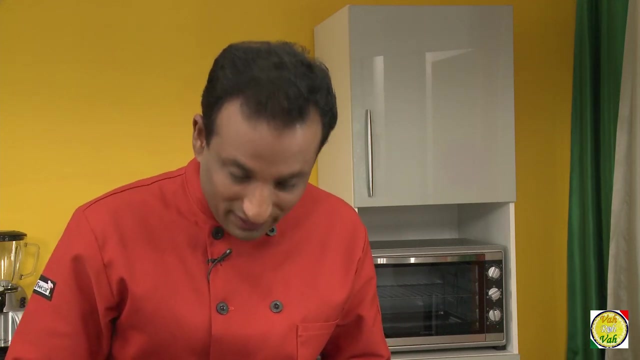 only give a very nice unique taste but also give thickening to this sauce. wow, look at it. and when you taste it it is got a tinge of sweetness also to this dish. but very, very nice, dear friends, look at this. now I'm going to flavor it with little of nutmeg, just. 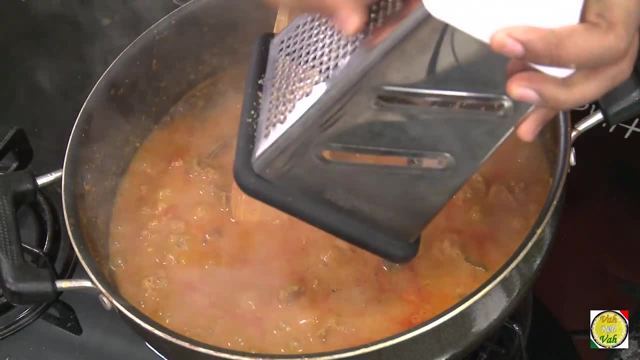 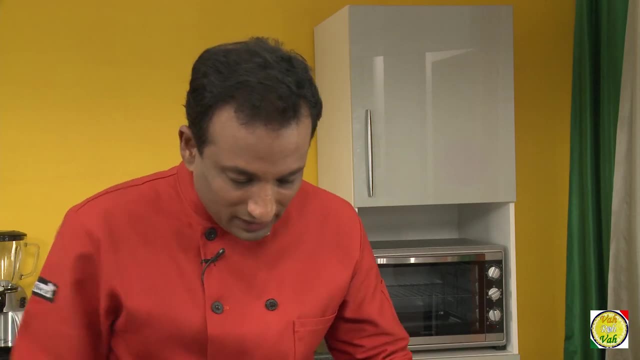 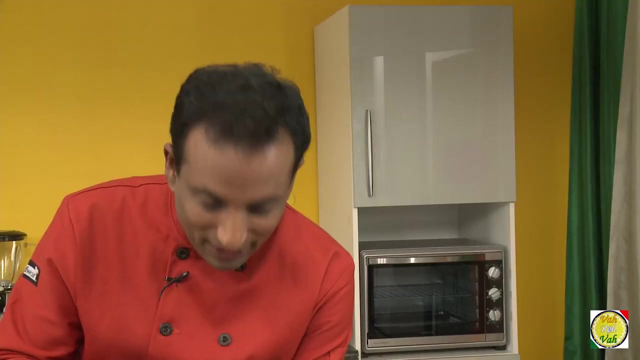 take that nutmeg and not too much. not too much nutmeg has a very strong flavor, so very little should be good enough. and then add a lot of chopped coriander in it. this is all cooked and switch off the flame and ready to be served.